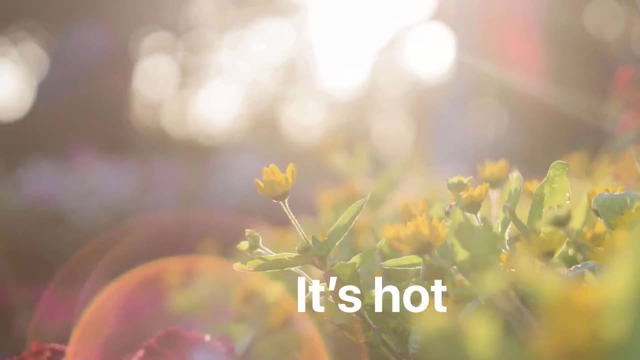 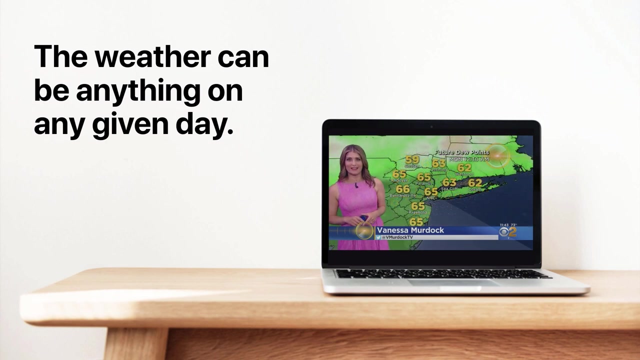 That too is the weather. Finally, it's hot today. That also describes the weather. Keep in mind: the weather can be anything on any given day, and while we do see patterns, which we'll talk about shortly, weather can fluctuate greatly. For example, in January in New York City. 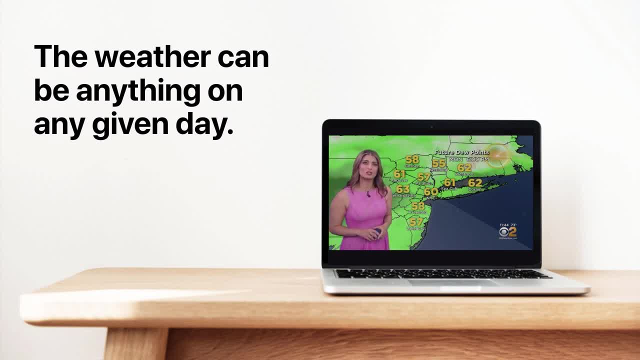 it's generally cold, But on any given day in January we could have seventy-five or eighty-degree Fahrenheit weather in New York. It would be strange, but that's the weather. It's a snapshot of what's happening right here, right now. 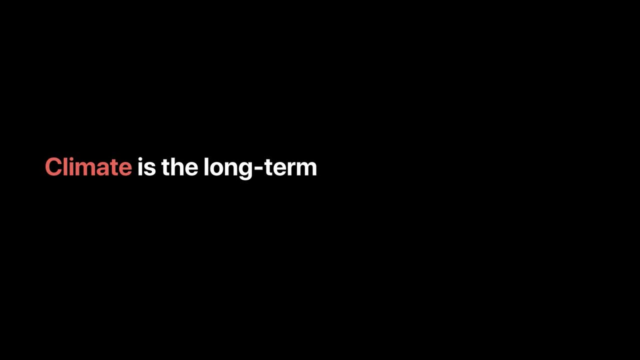 Climate, on the other hand, is the long-term average condition of the atmosphere for a location. The key here is that climate is long-term. It's a snapshot of what we expect to see in a location based on many years of data that has been accumulated and studied and averaged out. 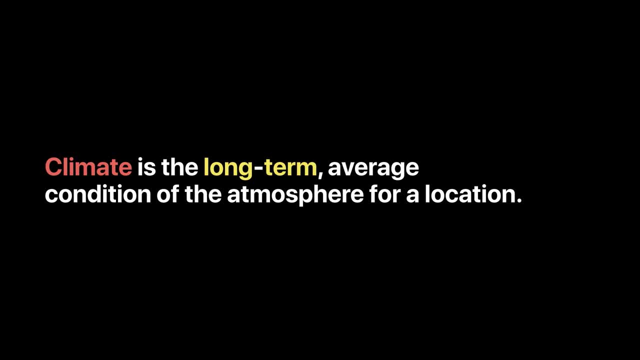 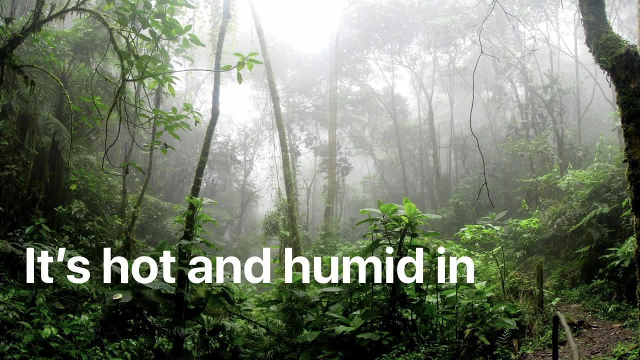 So it gives you a picture of what to expect for a particular location, though it's important to keep in mind that the day-to-day weather could be just about anything. Here are some examples of statements that describe the climate of a particular area. It's hot and humid in the Amazon. 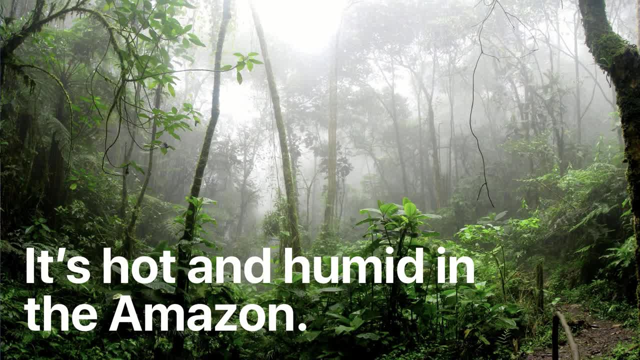 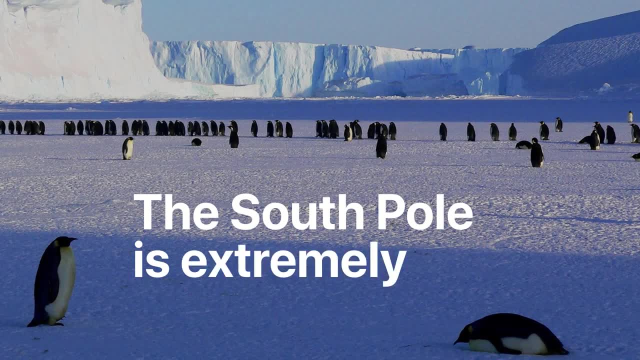 That's an example of climate. It's not always hot and humid in the Amazon, but on average that's what we expect to see there. Or if we were to say the South Pole is extremely cold and dry. Generally that's true, but certainly there are days where it's not true. 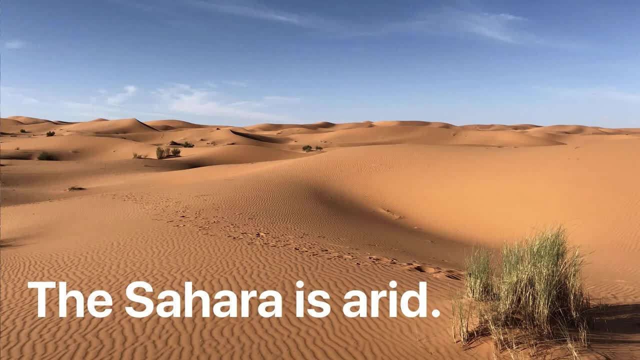 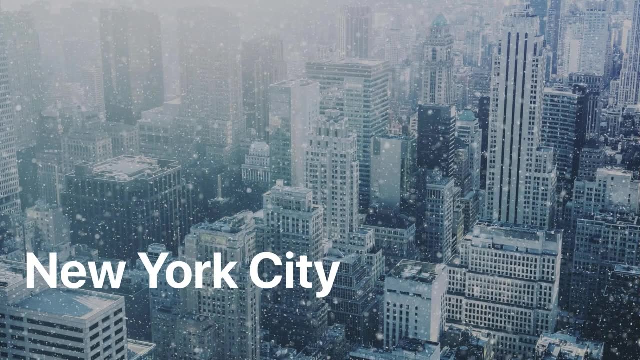 The Sahara is arid. Yeah, the Sahara Desert is generally very arid and dry, but it does rain there from time to time. New York City is cold in the winter Again, that's true, but we could have a warm day in January in New York. 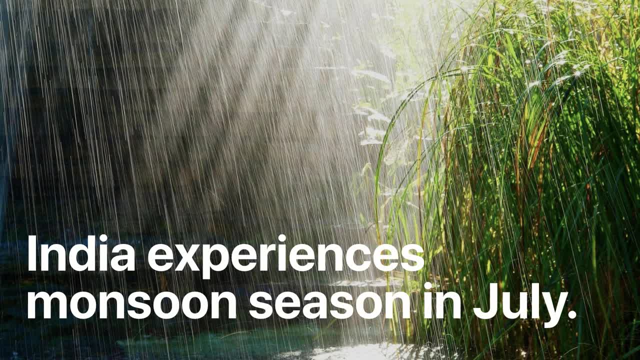 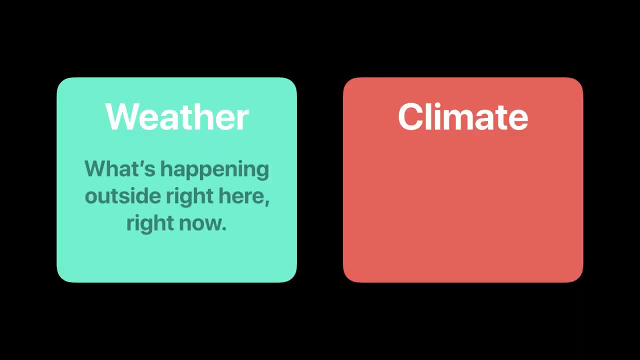 Finally, India experiences monsoon season in July. What that means is it usually is very wet and rainy in July in India, but that doesn't mean every minute of every day in July will always be wet. So to sum up, weather is what's happening outside right here right now. 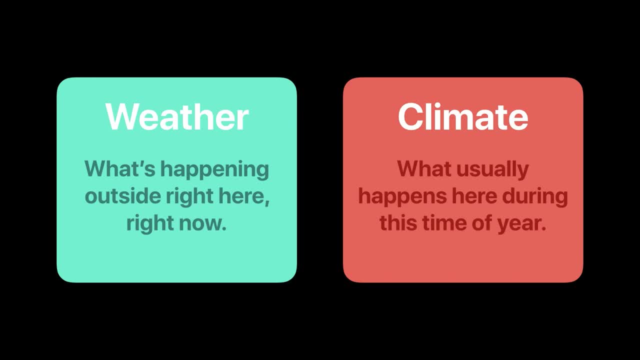 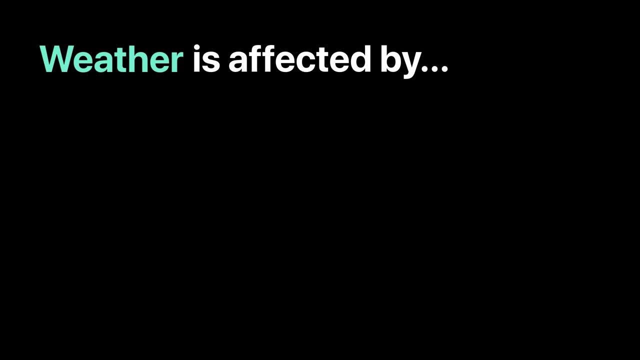 while climate is what usually happens here during this time of year, Now, weather is affected by a lot of different things. These are all different factors that give you a sense of what's happening in your location at this moment. These include things like the temperature, the wind, humidity, cloud cover, precipitation and air pressure.